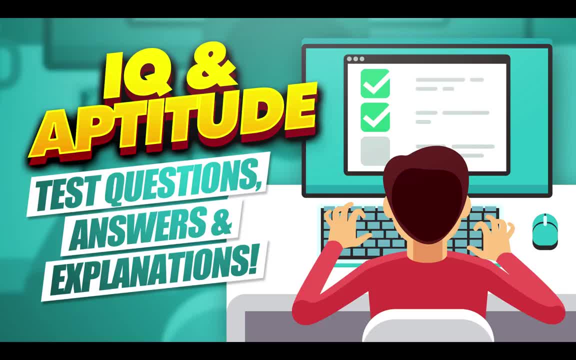 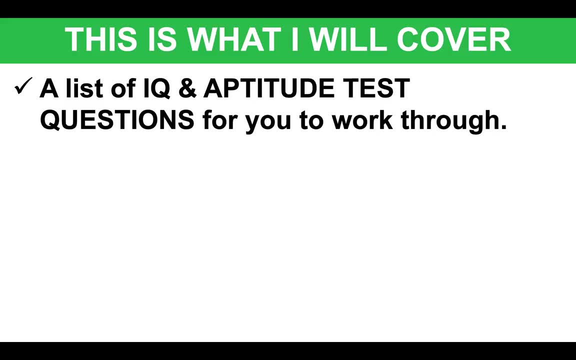 fully, from start to finish, because I will help you to increase your scores significantly and to achieve that goal. This is what I will cover. I will give you a list of IQ and aptitude test questions for you to work through live on the screen. I will give you tips on how. 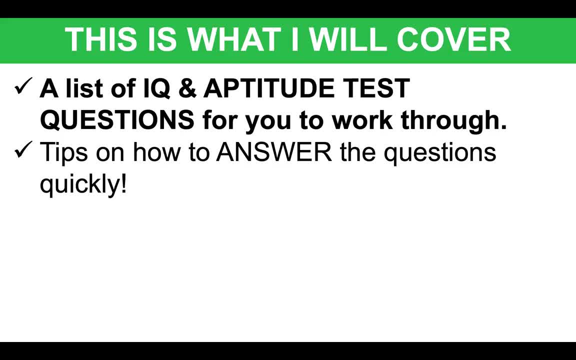 to answer the questions quickly, and that must be our goal. We want you to be able to tackle the questions in as fast a time as possible, because that will help you to pass your test. I will also give you answers to the questions and full explanations, And I 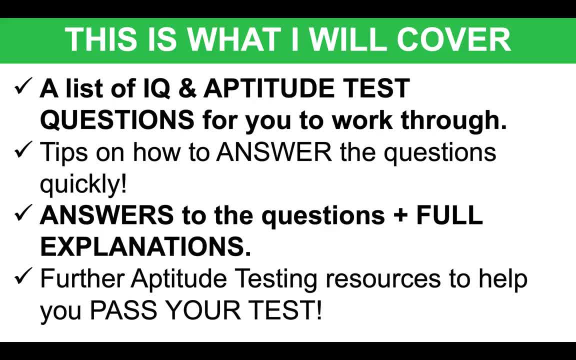 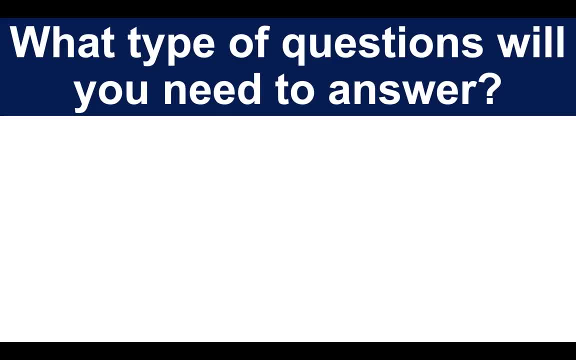 will also tell you about further aptitude testing resources you can get access to to help you pass your job test. So there's four reasons why you should stay tuned Now. first of all, what type of questions will you need to answer during your IQ and? 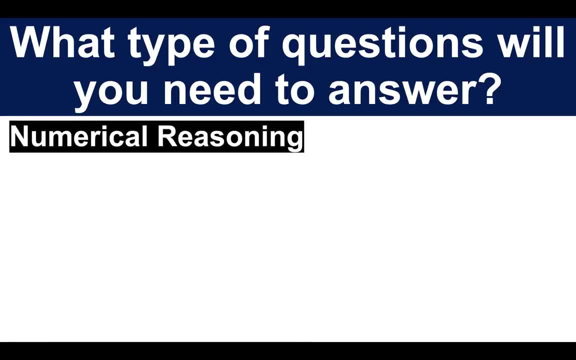 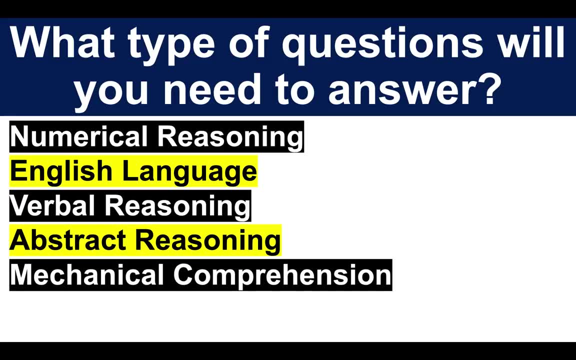 aptitude test. Well, you will need to tackle numerical reasoning test questions, English language test questions, verbal reasoning, abstract reasoning test questions and mechanical comprehension test questions too. So there's five different categories there that we are going to work through together today on this video And to help you make progress. I'm 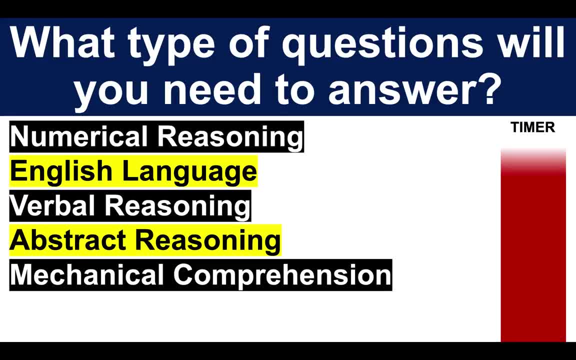 going to get you to answer the questions under today's video. I'm going to give you a strict timer and I want you to stick to it as much as possible as we progress through the questions. So the first category is numerical reasoning. Let's 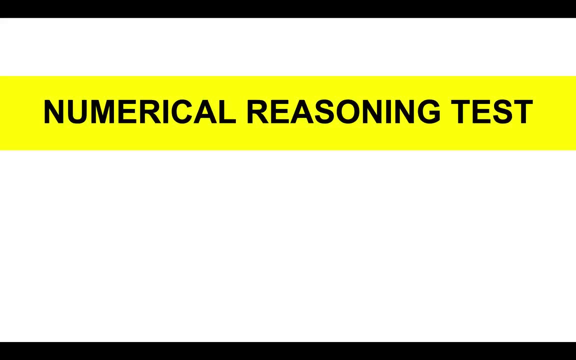 start working through some numerical reasoning test questions. I will put up a question on the screen, I will work through it with you in a slow pace and then I will get you to try one so that you are making progress. Question number one: What is 25% of 80?? So it's a very 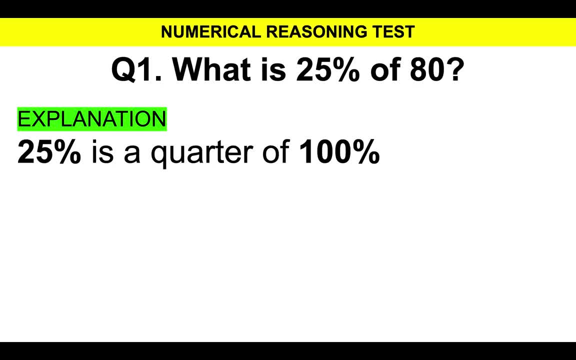 simple one to start off with. The explanation to that is: 25% is a quarter of 100%. Therefore, to get the answer, all we need to do is do the calculation 80 divided by 4, because that's 25%, and that gives us. 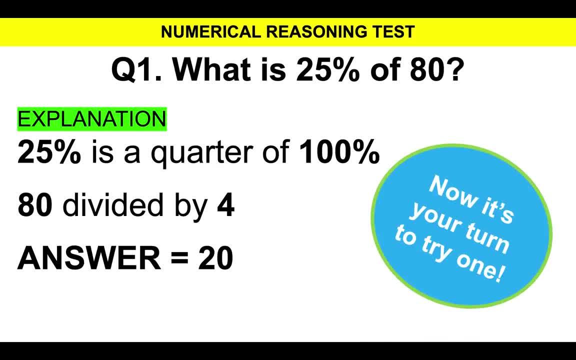 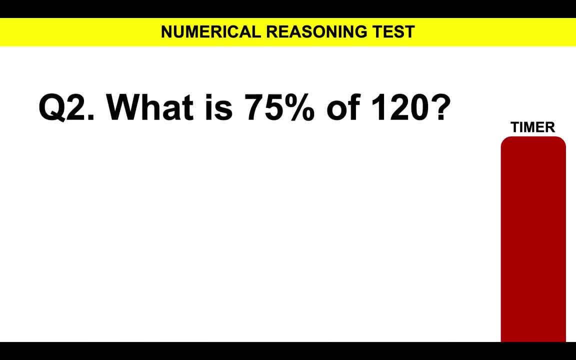 the answer of 20.. Now it's your turn to try one similar to this question. I'll put the question up on the page and there's a timer for you to work to Question number two. What is 75% of 120?? 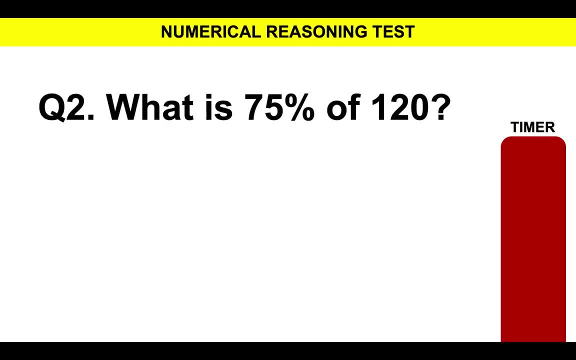 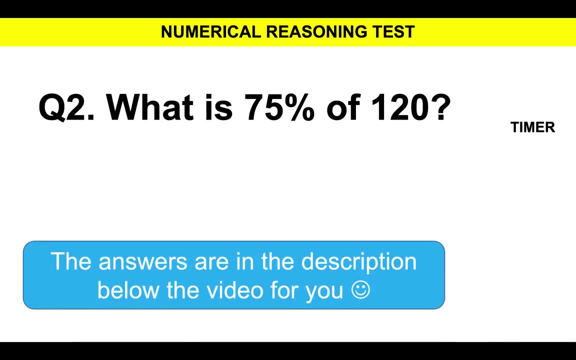 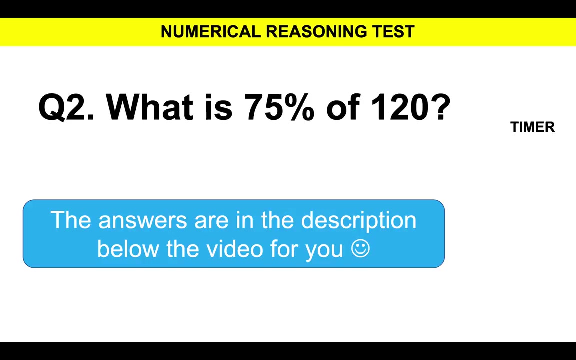 And you have the time. it takes that timer to go to the bottom to come up with your answer. Here we go. Excellent, Well done, And I have put the answers to the questions in the description below the video for you, So check them out as you work through each of the questions. Now that 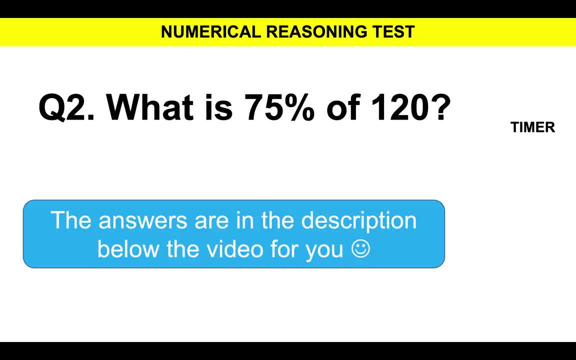 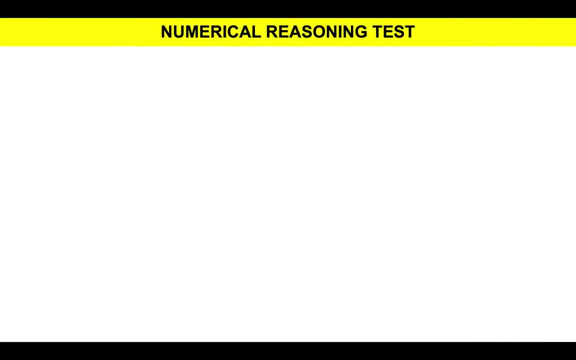 gives you a little bit more time than that in your real IQ and aptitude test, And if you find you need to pause the video to have more time, that is absolutely fine. And if you want to use a calculator too, you can do. Question number three: What is four-fifths? 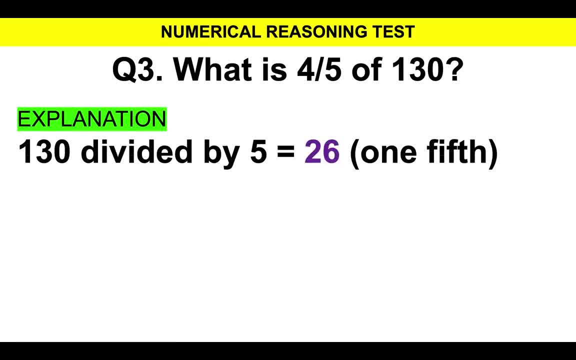 of 130?? Here's my explanation. So 130 divided by 5, which would be one-fifth, equals 26.. So if 26 is one-fifth, we need to then multiply that by four to get four-fifths. So the answer: 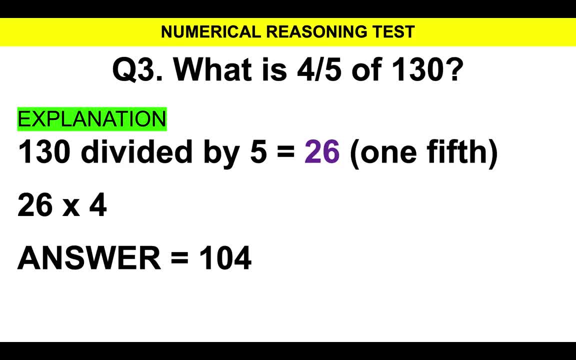 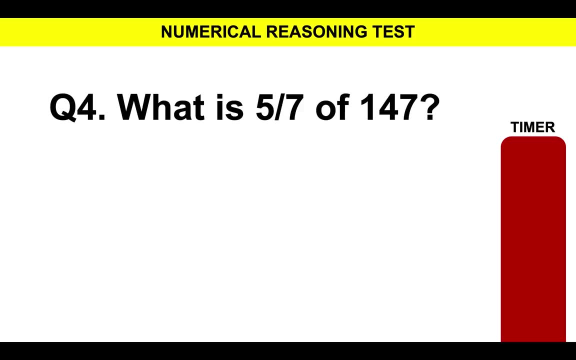 is 140.. And these are the kind of questions- once we become proficient in tackling them, we can gain really easy, quick marks during our IQ and aptitude test. So now it's your turn to try one similar to this, Question number four. Here we go. What is five-sevenths of? 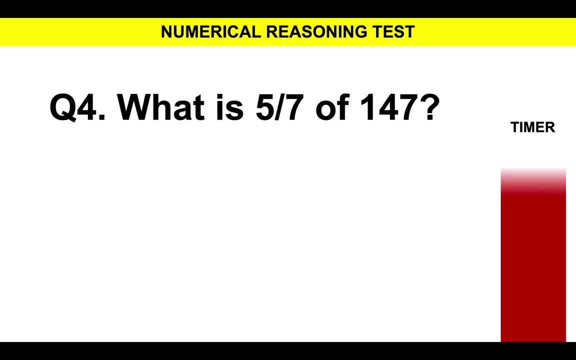 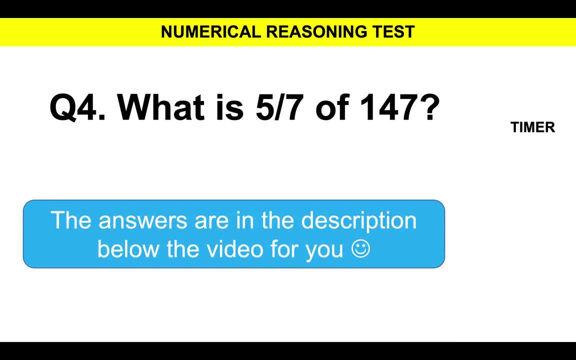 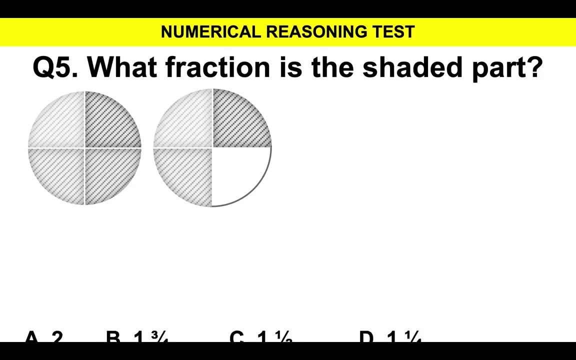 147? There's a timer, Excellent. So again, the answers are in the description below the video for you. Question number five: What fraction is the shaded part? Is it A, 2, B, 1 and 3 quarters C, one and? 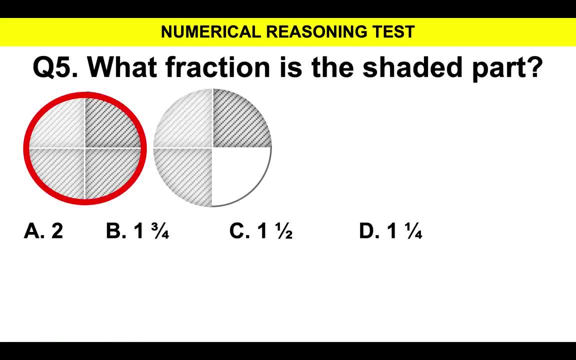 a half, D one and a quarter. So if we start on the left we can see that shaded part. there is four quarters. OK, so that makes up one Four out of four And on the other one is three quarters. 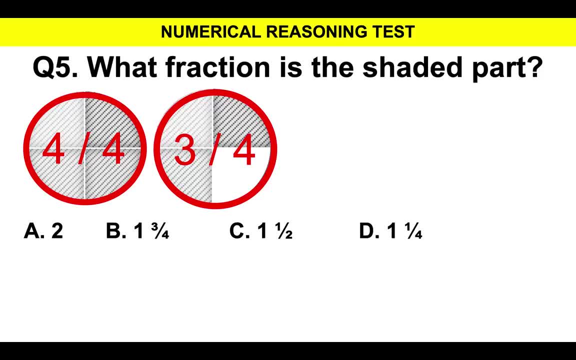 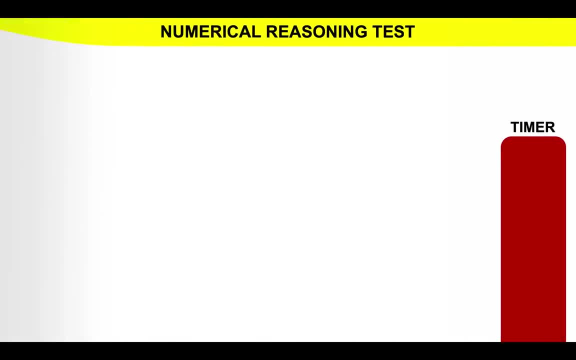 three shaded parts out of four, so that's three quarters. The correct answer, as we add those together, is B, one and three quarters. Very simple. Now it's your turn to try one Question, number six: What fraction is the shaded part? Is it A, three and a quarter? 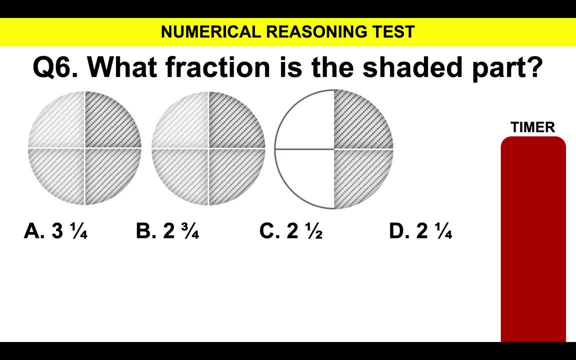 B two and three quarters, C two and a half Or D two and a quarter, And you have the time It takes the timer to go to the bottom to come up with your answer. Brilliant Well done And, as I said before, the answers are in the description below the. 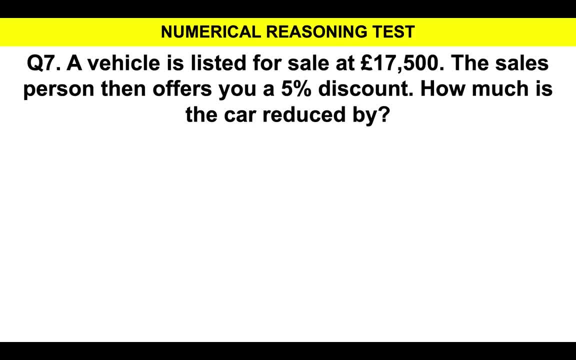 video for you. The next question, number seven. Let's make it a little bit more difficult. A vehicle is listed for sale at 17,500 pounds. The salesperson then offers you a 5% discount. How much is the car reduced by Now? this is the important. 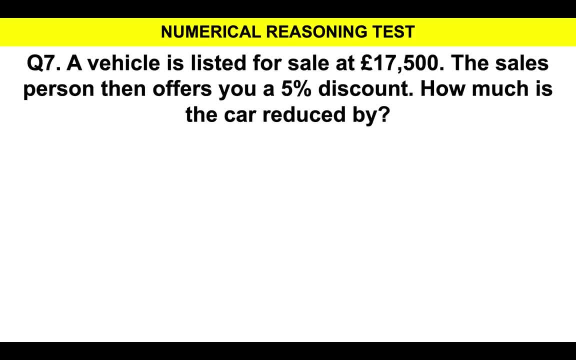 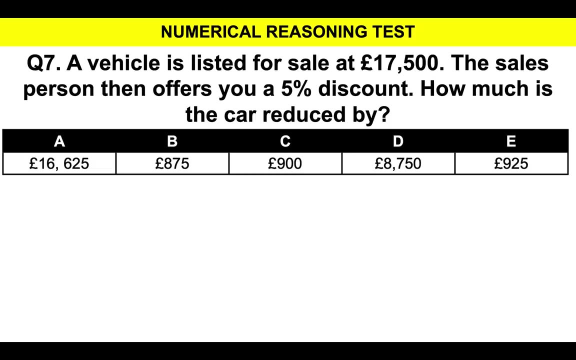 thing- Don't make the mistake that a lot of people do is not reading the question correctly. That last bit is important. How much is the car reduced by? Not how much does the car cost, but how much is it reduced by? Is it A 16,625?, B 875?, C 900?, D 8,750? Or E? 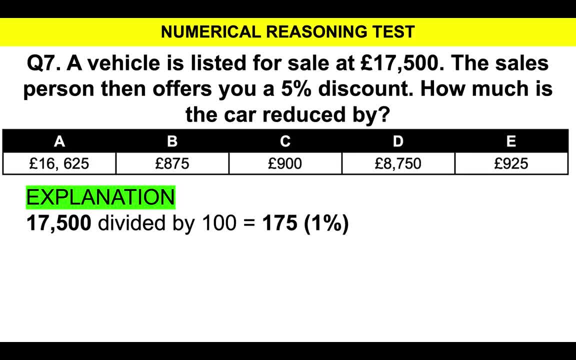 925?. So to calculate this…. 19,500 is the list price Divided by 100, to get 1% is 175.. We then multiply 175 by 5 to get the 5% discount. So therefore the answer is 875.. Don't forget to read the question. 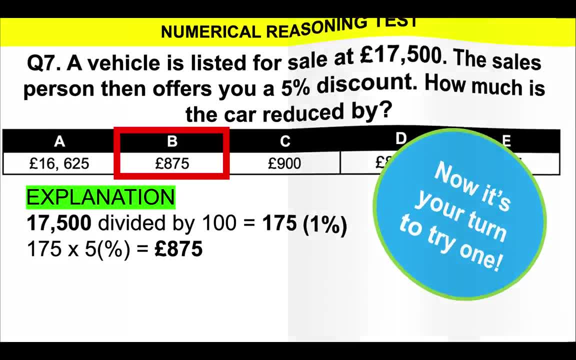 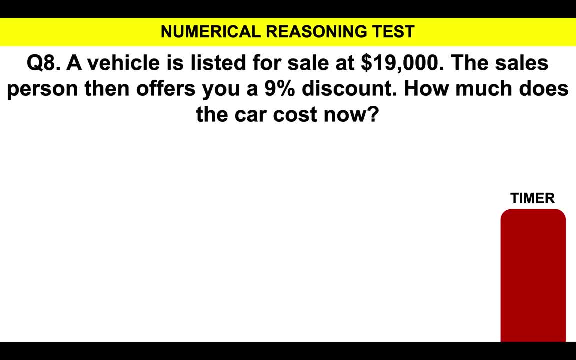 Very important. So now it's your turn to try one, and make sure you read the question. Here we go. Question 8. A vehicle is listed for sale at $19,000.. The salesperson then offers you a 9% discount. How much does the car cost now? 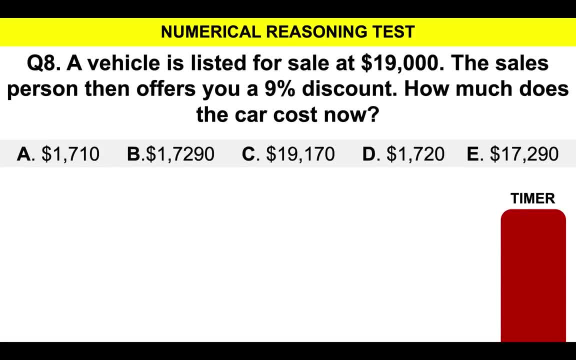 Now, with the 9% discount taken off, is it A $1,710?, B $1,729?, C $19,170?, D $1,720? Or E $17,290?. Here's the timer. 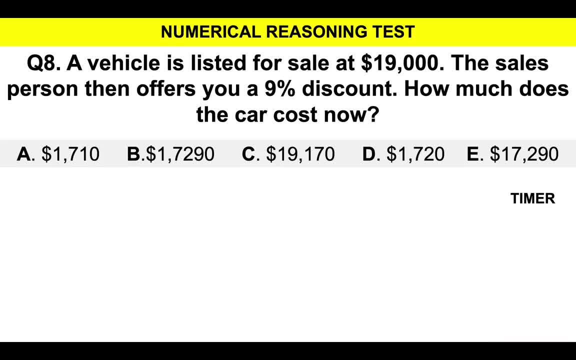 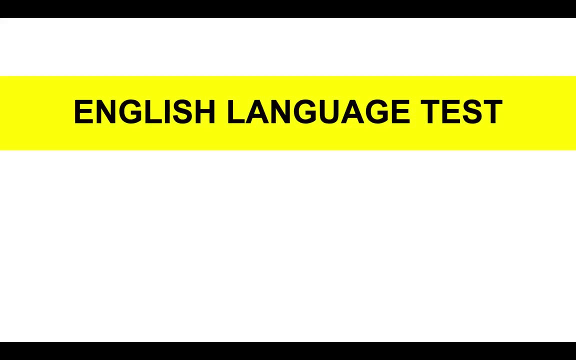 Excellent. I hope you're enjoying these. Please don't forget give the video a LIKE if you're enjoying it. I appreciate your support. Don't forget to SUBSCRIBE. Thank you, Let's now move on to English language test questions. Question number nine: Which one of the following: 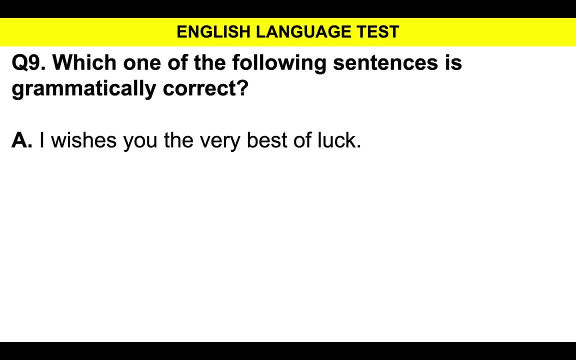 sentences is grammatically correct: A- I wishes you the very best of luck. B- Our holiday has been postponed. C- The government is implementing a new law today, Or D. It is difficult to understood my teacher. Well, if we break them down, we can see that. I wishes you the 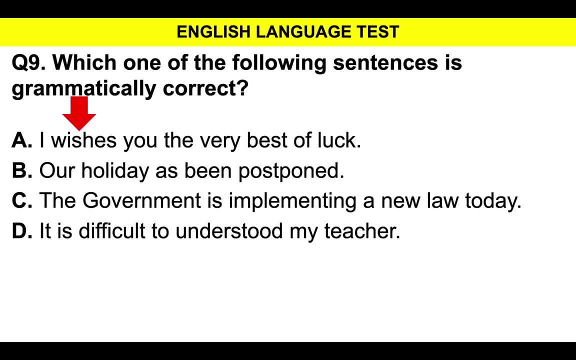 very best of luck is not grammatically correct. It should be. I wish you the very best of luck. Our holiday has been postponed. That's wrong. It should be. our holiday has HAS And D. It is difficult to understood. my teacher is not grammatically correct. It should be it. 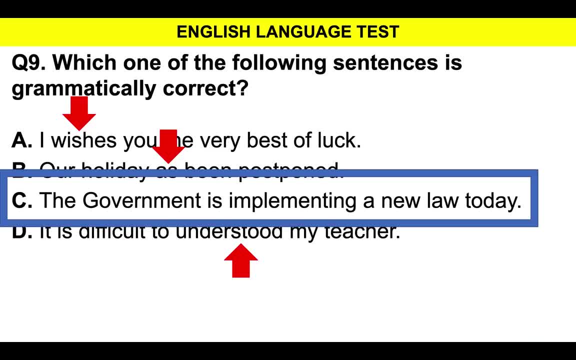 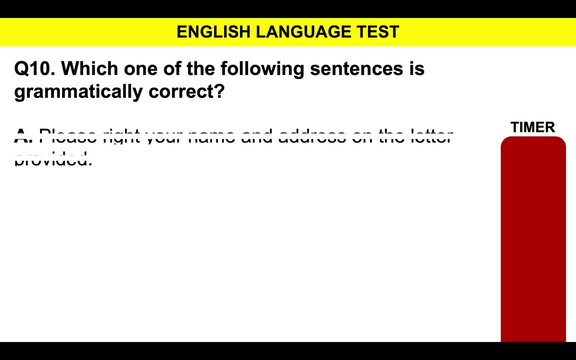 is difficult to understand, my teacher. Therefore, the correct answer: The government is implementing a new law today. C is the correct answer. Now it's your turn to try one similar to this English language test question, Question number 10.. Which one of the following sentences is grammatically correct? A, Please write. 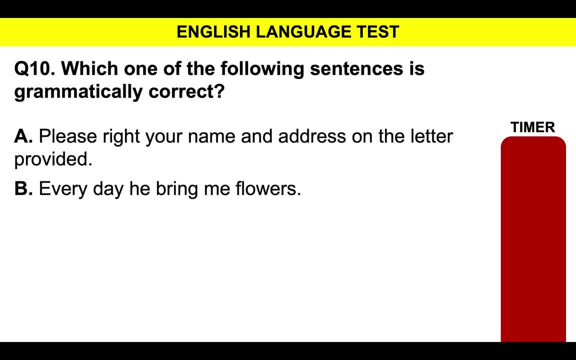 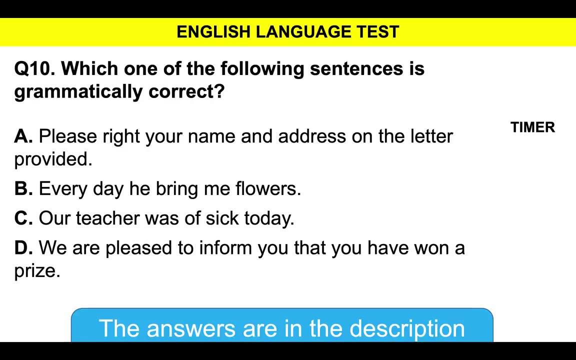 your name and address on the letter provided. B. Every day he bring me flowers. C. Our teacher was off sick today. D. We are pleased to inform you that you have won a prize. Here's the timer. Fantastic, And don't forget. the answers are in the description below the video for. 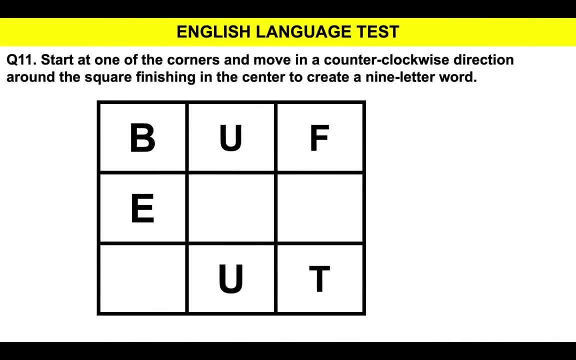 you Question number 11.. This one's a little bit more fun. We have to start at one of the corners and move in a counterclockwise direction around the square, finishing in the center, to create a nine letter word. So we can start at whichever corner we want to, And we have 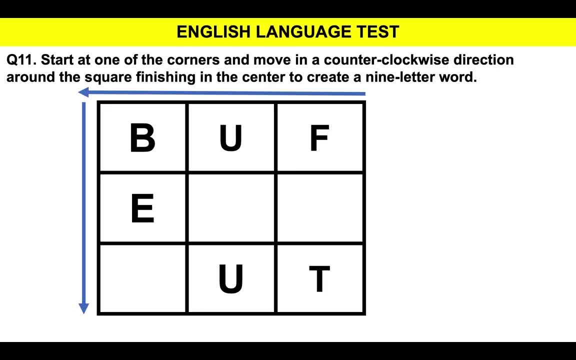 to go counterclockwise, Which is that way You don't ever have to calculate or carry out any questions with clockwise or counterclockwise or anticlockwise. Clockwise is the direction the hands will go on a clock. Counterclockwise. 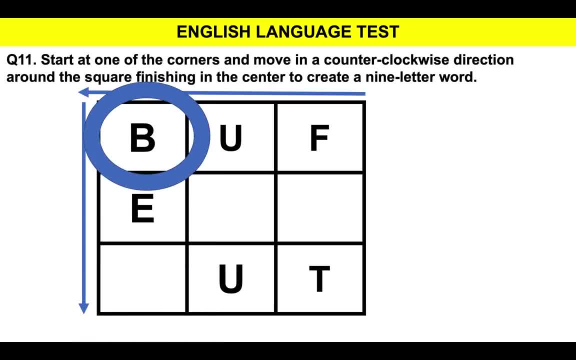 or anticlockwise is the other direction. So if we start with B and then go counterclockwise, we can add an A there, an I there and an L there And we get the word BEAUTIFUL finishing off in the center to get that nine letter word BEAUTIFUL. So this is quite difficult. 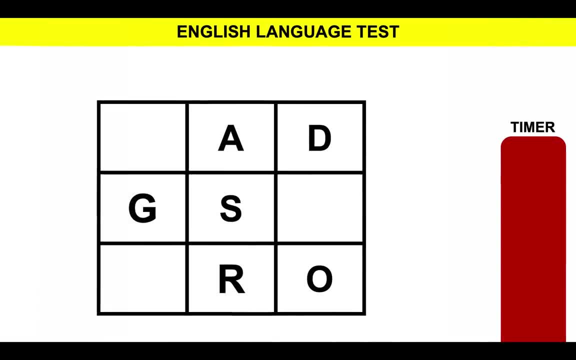 It seems easy, but it's not. So now it's your turn to try one Question, number 12.. Start at one of the corners and move in a counterclockwise direction around the square, finishing in the center, to create a nine letter word. You have the time. It takes the timer. 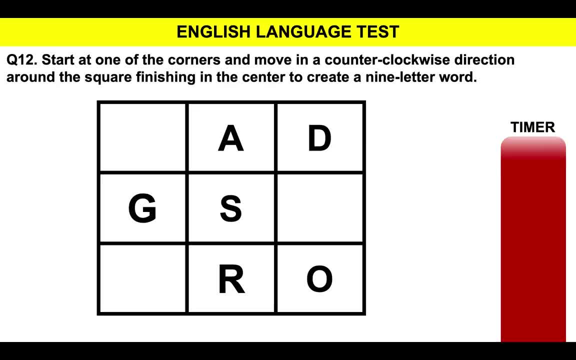 to go down to choose your nine letter word. Here we go, Fantastic, And, as I say, the answer is this one. It's a good one, It's the J, J, Y and J. There we go, Fantastic, And, as I 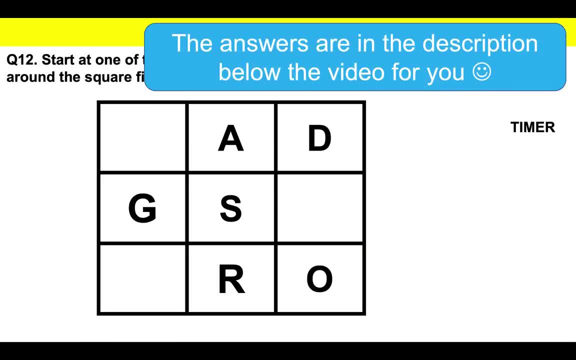 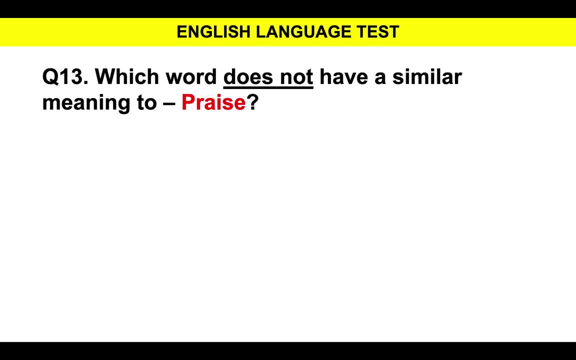 I said, the answers are in the description below the video. And don't forget to subscribe. Thanks, answer is in the description below the video for you. Brilliant question, Number 13.. Which word does not have a similar meaning to PRAISE? A Recognition, B, Appreciate, C- Plaudit? 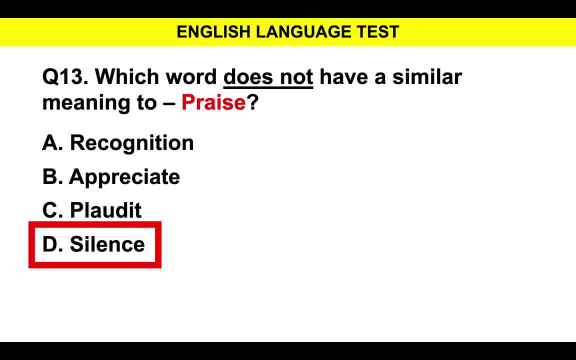 D Silence. The correct answer is silence, because praise is similar to recognition. It is to appreciate and to plaudit. But D Silence does not have a similar meaning to praise. So now it's your turn to try one of these. Here we go. Question number 14.. 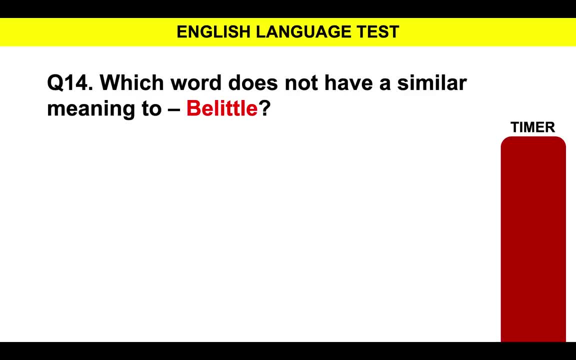 Which word does not have a similar meaning to BELITTLE A, Criticize, B, Downgrade, C, Overrate, D, Discredit? Again, you have the time. It takes the timer to come up with your answer. Here we go. 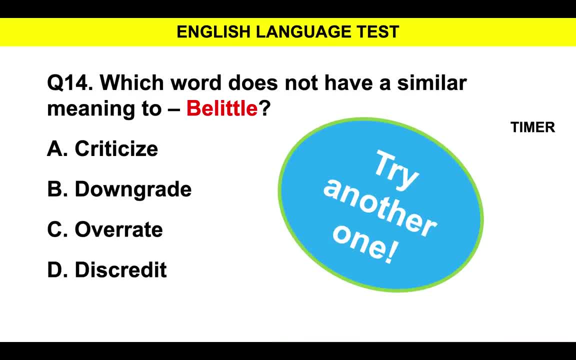 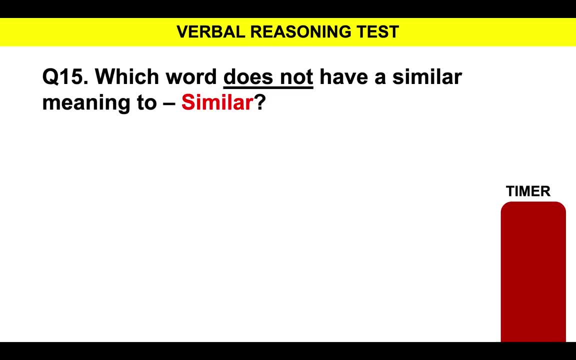 Awesome, Fantastic. Try another one of these, Let's see how you get on with another one, Question number 15.. Here we go. Which word does not have a similar meaning to SIMILAR A, Akin, B, Coincidental, C, Resembling, D, Contrasting? Here's the timer. 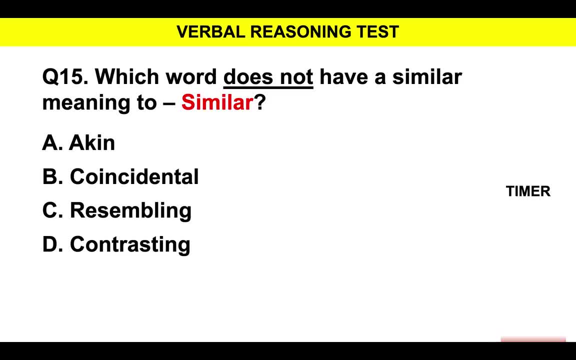 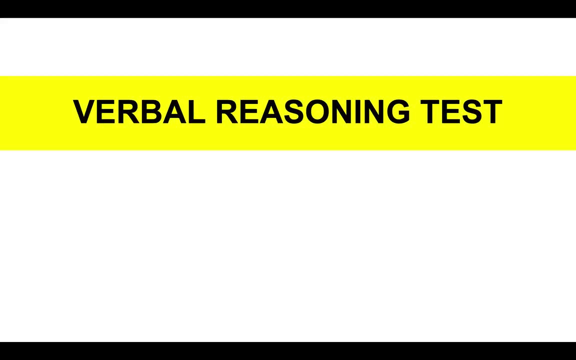 Well done And I think, the important thing. before just quickly we move on to verbal reasoning test questions. The important thing to remember is the way to get good at these IQ and aptitude test questions is to carry out lots of practice, And I will tell you soon where you can get. 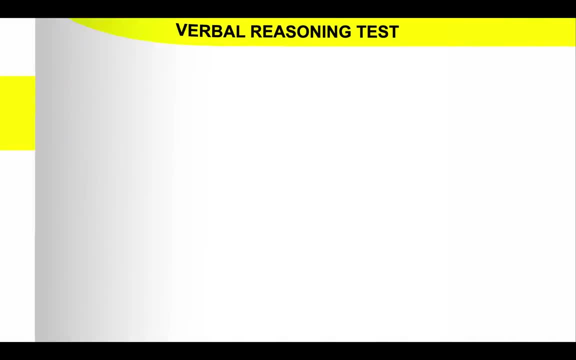 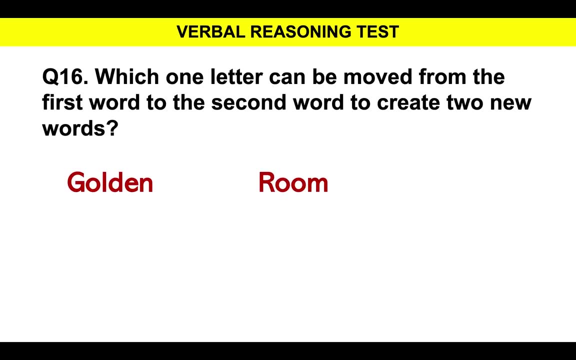 more practice. once we've worked through the remainder of these verbal reasoning tests, Let's take a look. Question 16. Which one letter, Which one letter can be moved from the first word to the second letter, The second word to create two new words, So which one letter can be moved from the first? 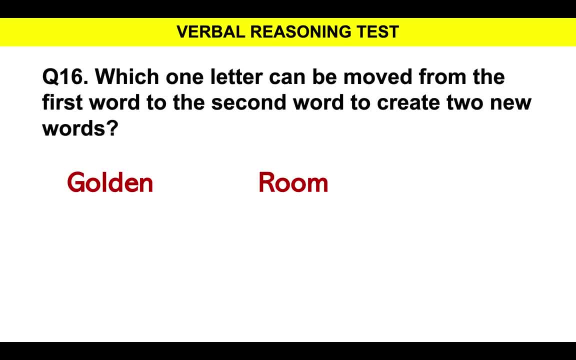 word golden to the second word room to create two new words. So if we move the G over to the right we get the word groom and we also get the word olden. So we're just moving one word, one letter, from the left word to the right to create two new words. I hope that. 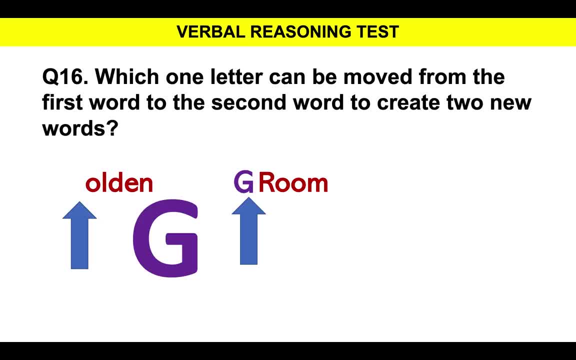 makes sense And the correct answer there is G. So now it's your turn to try. Go on, Here we go. Question number 17.. Which one letter can be moved from the first word to the second word to create two new words? Which letter will you choose? Here's a timer. 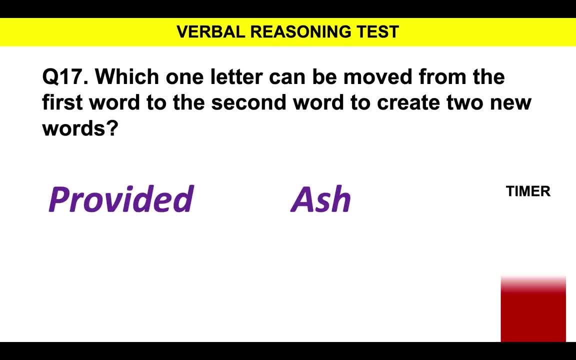 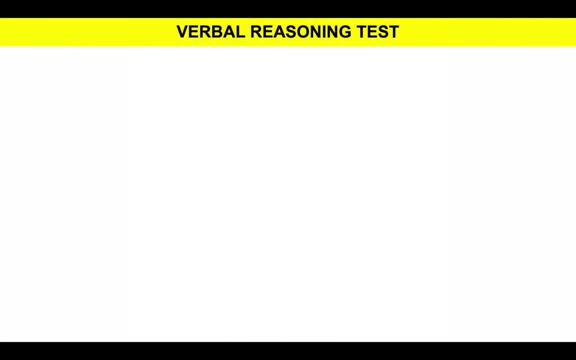 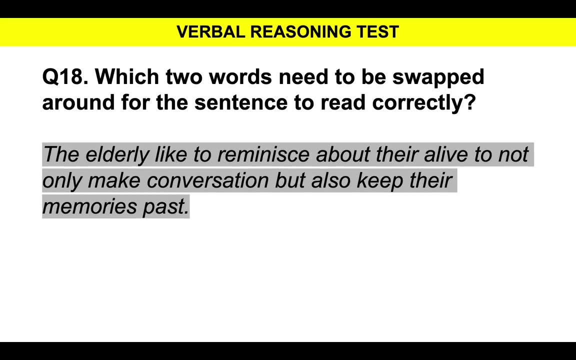 Brilliant. Here we go with another one, Question, number 18.. Which two words need to be swapped around for the centre To read correctly? Which two words need to be swapped around for the sentence to read correctly? The elderly like to reminisce about their alive, to not only make conversation. 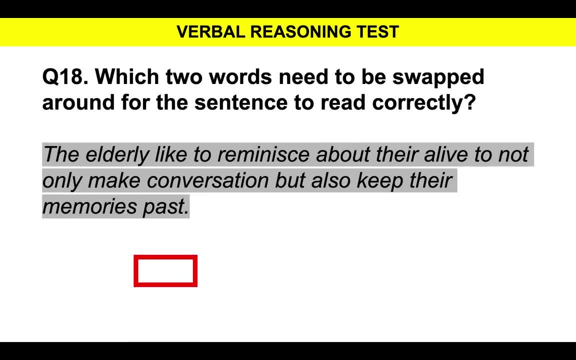 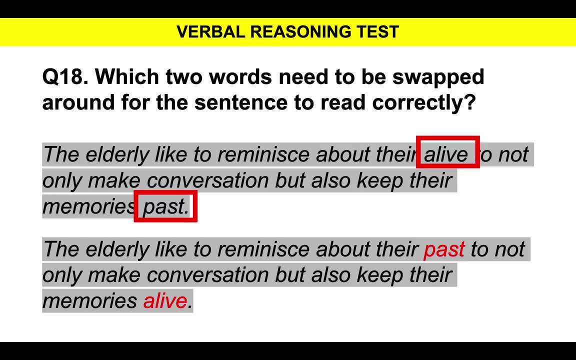 but also keep their memories past. So if we move around past and alive, we get this. The elderly like to reminisce about their past, to not only make conversation but also keep their memories alive. So now we have a correct sentence. Here's your turn. Have a go at this. 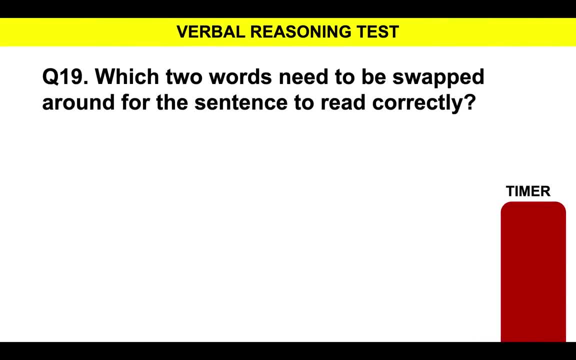 next one, Question number 19.. Which two words need to be swapped around for the sentence to read correctly? Michael correctly fitting his safety harness after began his descent of the mountain. Choose your two words. Here's a timer, Excellent, Well done, And I hope you can see by working through lots of practice test questions. 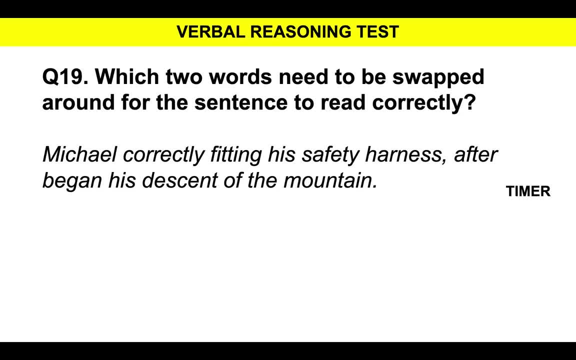 it's not only a question, it's a response. It's a response to a question. It's a response to a question. It's not only fun, but you will get better at them, because these type of questions will come up during your IQ and aptitude test. Let's have a look at another one. Which one? 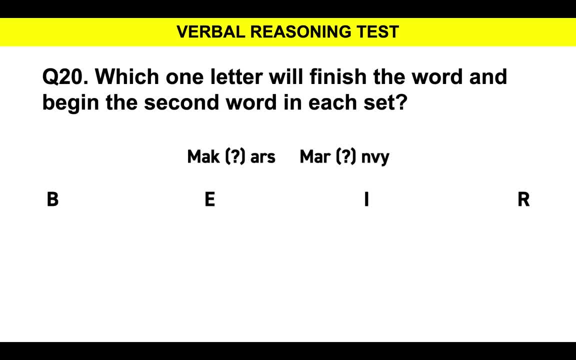 letter will finish the word and begin the second word in each set. So which one letter, B E, I, R, will finish the word and begin the second word in each set. We have to decide which one letter from BEIR goes there and there to finish the first word and then start. 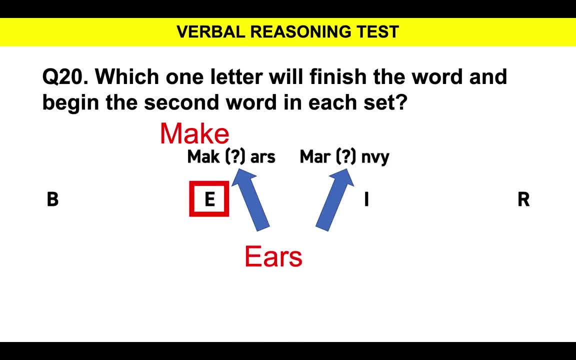 the second. Well, I think that's good. If you have a sound mind, then you have a sound mind. You'll get better at them. It's challenging, but maybe because sometimes you'll have a, we would have the word there: MAKE and EARS and MARE and ENVY, Simple. So now it's your turn to 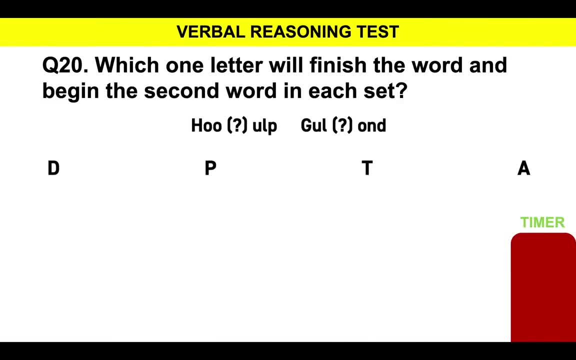 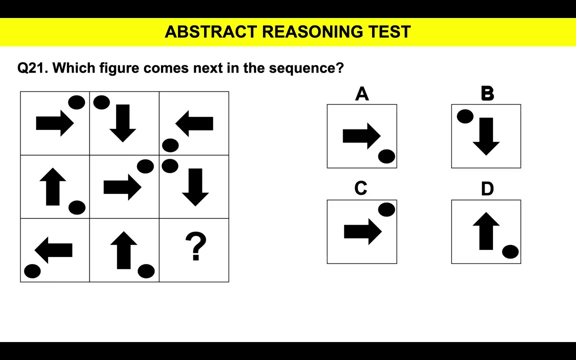 try one. Here we go, Question number 20.. Which one letter will finish the word and begin the second word in each set? Is it D, P, T or A? Here's a timer Brilliant. Let's now move on to abstract reasoning test questions. Here we go, Question 21.. Which? 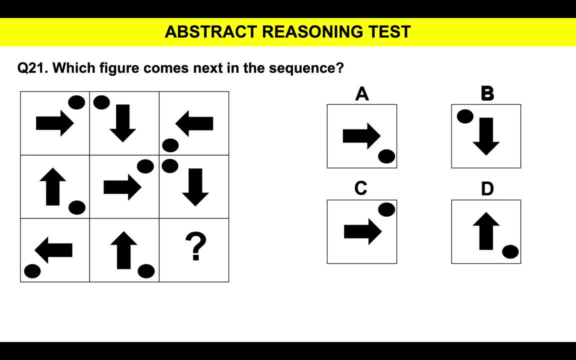 figure comes next in the sequence. So on the left hand side we have nine squares, all with different shapes, and we have to work out from A, B, C and D on the right which one goes there. It looks very confusing, but there is a logical process for working out. 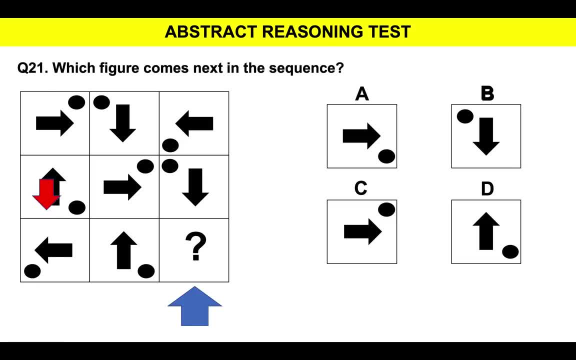 abstract reasoning test questions. All you have to do is start at the top left, Pick one shape and then have a look for a sequence. So if we look at that black arrow which is pointed to the right, it then moves 90 degrees south. It then moves to the west. 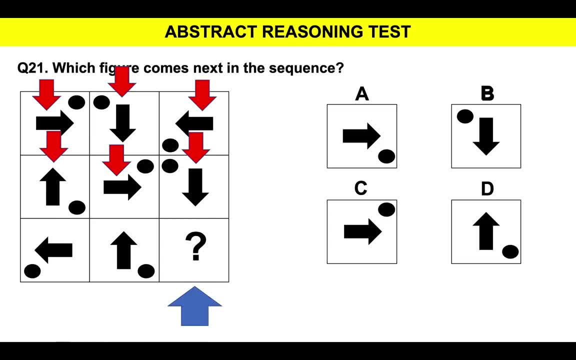 It then moves north, It then goes east, It then goes south, And it keeps rotating 90 degrees clockwise. So where the question mark is there, that's where it will need to be Now. this is an important tip. All you need to do quickly, then, is look at your answer. 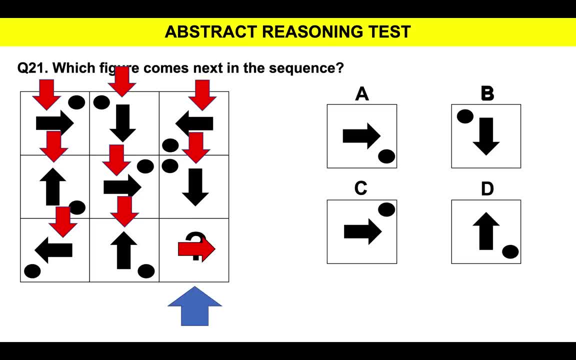 options A, B, C and D And see which one doesn't have an arrow pointing to the right and then eliminate that answer option. So B is pointing down, D is pointing up. We can eliminate those. So it's either. 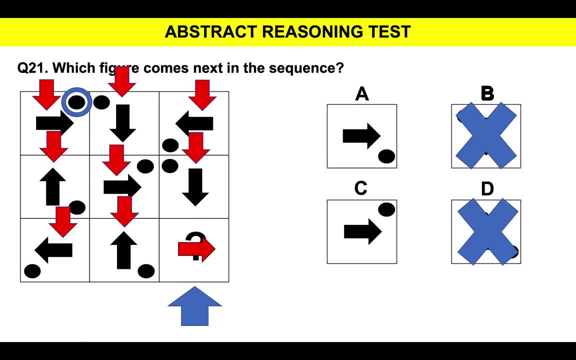 A or C. Now all we need to do is choose the other shape within each square, And this time it's a black dot. So it starts at the top right and then it moves anticlockwise to the top left, and then anticlockwise to the bottom left, And it moves around the square each. 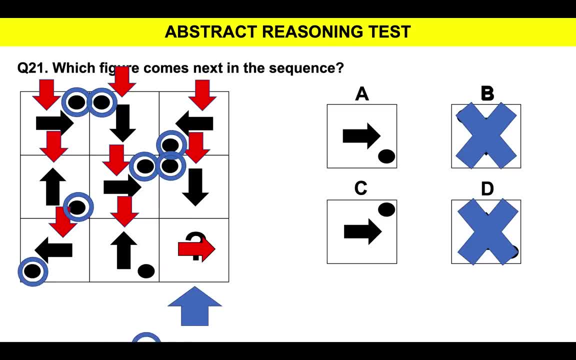 time, anticlockwise, 90 degrees. So therefore, in the shape we are looking for in the sequence, it would go there. That's not A. The correct answer is C. So you can see, by following a logical sequence we can. 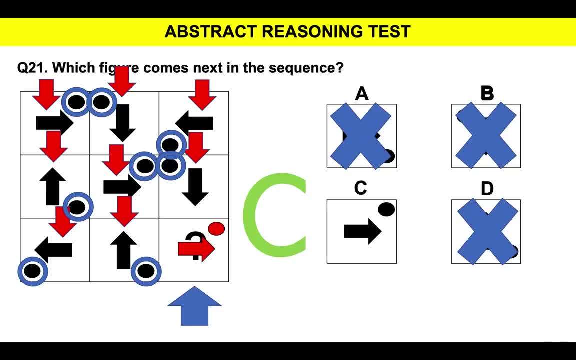 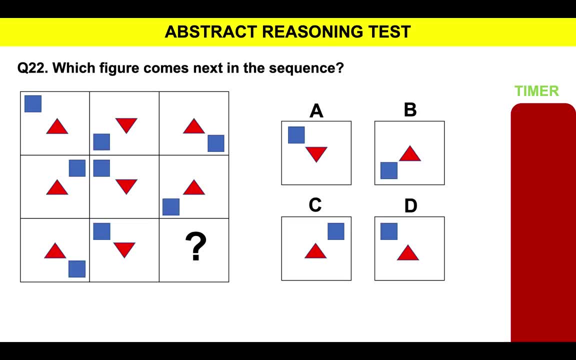 come up with the right answer, We can eliminate which ones are not correct. So now it's your turn to try one. Here we go, Question 22.. Which figure comes next in the sequence A, B, C or D? And you have the time- it takes that timer to go down- to come up with your. 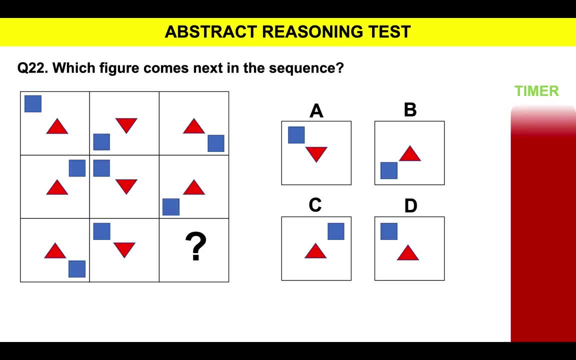 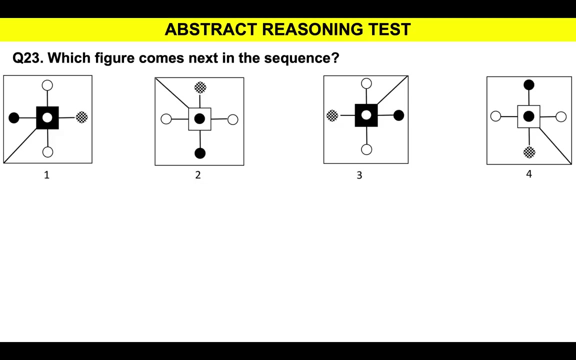 answer. Here we go. Brilliant, Well done, Fantastic. If you are still with me, I'm really proud of you. You're making excellent progress. Keep sticking at it, because your scores will improve. Here's another one, Question 23.. Which figure comes next in the sequence? So we have one, two. 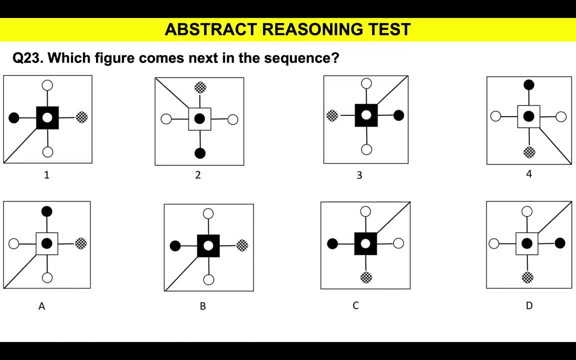 three, four. We have to decide which one would come next in the sequence from the answer- options A, B, C or D- And when we first look at these shapes and patterns, they are confusing. But if we break it down in a simple process, we can easily answer the question. So pick. 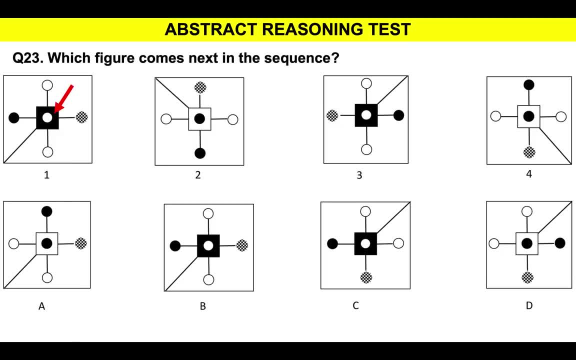 one part of the shape from the top. I'm going to go with the middle part And you can see we have a black square with a white circle in the middle And as we progress it then alternates to a white square with a black dot. It then goes back to the black square. 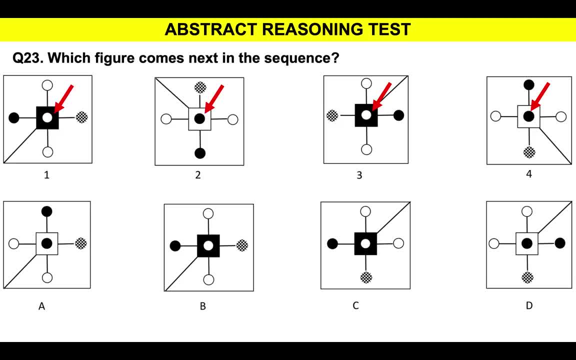 with the white dot, And then it goes back to that there. So in the sequence, we are looking for one that has a black square and a white dot, because that's the sequence. A doesn't have that, So we can eliminate it, And D doesn't have it either, So we can eliminate. 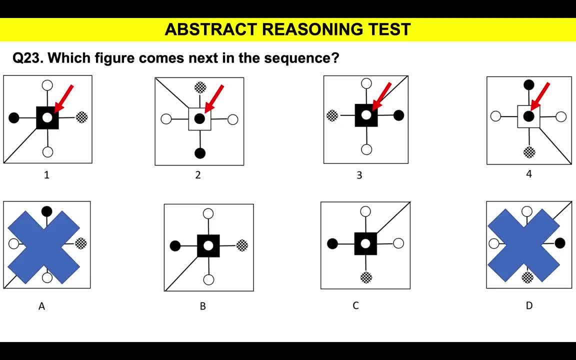 that as well. So it's either B or C. Now all you need to do is choose another one element of the shape and we will go for that checkered circle. And if you notice, as the sequence progresses, it moves counterclockwise 90 degrees. So it goes to the top, It goes to the north. 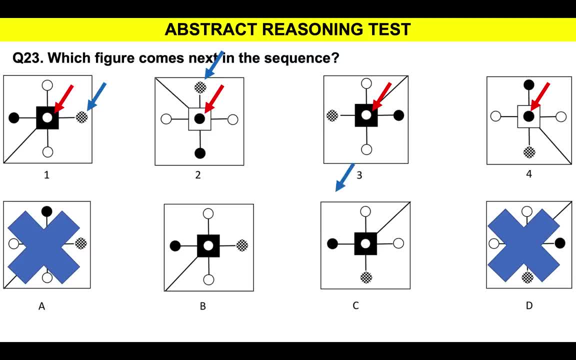 So it starts off on the east, It goes to the north, It then goes to the west, It goes to south. So we then need to find one which is in that location back at the start. So it's not C, because that's pointing south. Therefore, the correct answer is B, And you can see that. 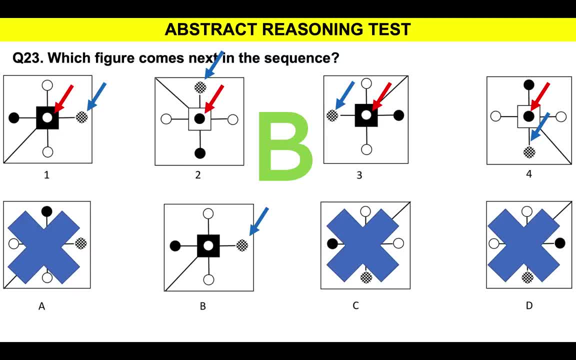 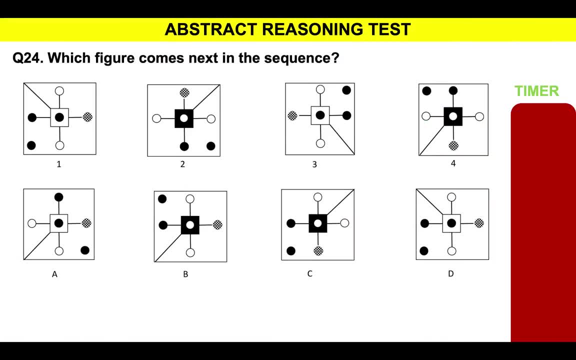 by practicing these questions and using a process of elimination, you can quickly come up with the right solution. So now it's your turn to try again. An abstract reasoning test question. Here we go, Question 24.. Which figure comes next in the sequence, A, B, C or D? And you have the time it takes the timer to come down to. 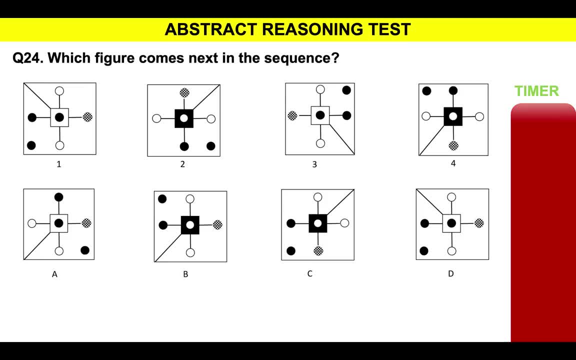 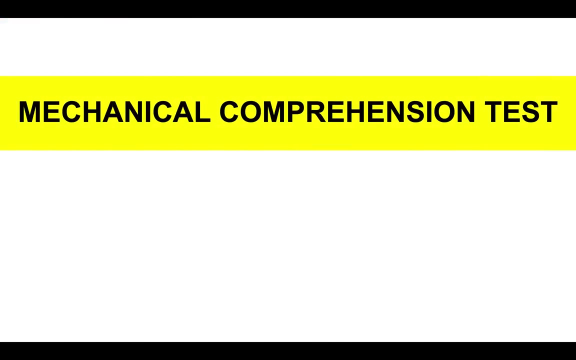 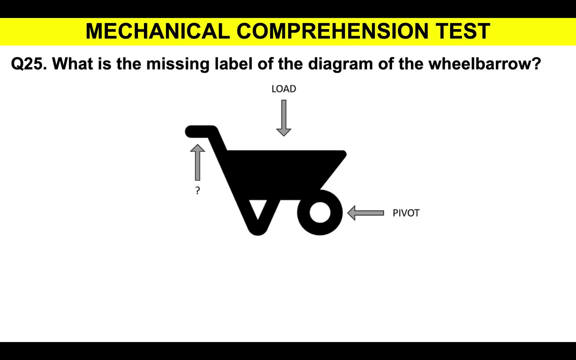 the bottom to choose your answer. Here we go. Fantastic, Well done. OK, Let's take a look now at a mechanical comprehension test question. Question is question 25.. What is the missing label of the diagram of the wheelbarrow? So, 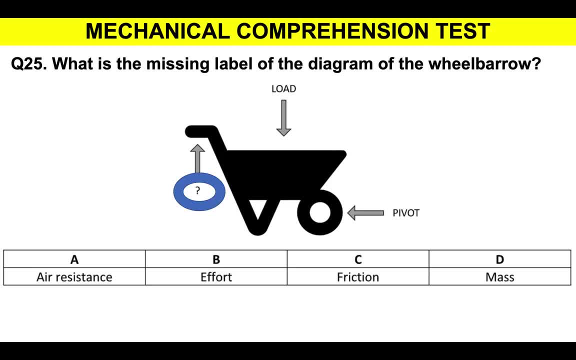 we are looking for that missing label there Is it: A air resistance, B, effort, C, friction, D, mass. Well, we can see that we've got the load which is going downwards, because the load will be in the wheelbarrow. We have the pivot there, which is the wheel. So which? 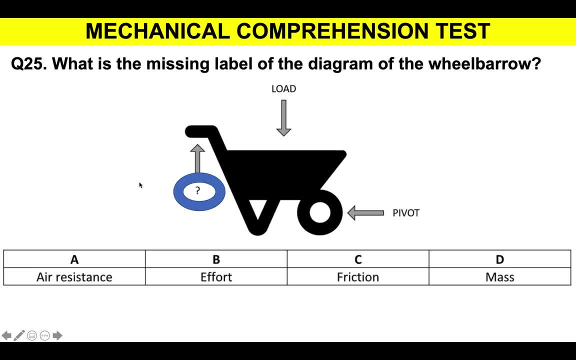 word, which label goes there? If you think about it, you would have to lift the wheelbarrow, and that takes effort to lift it up. So the correct answer, the logical one, is effort B. So now it's your turn to. 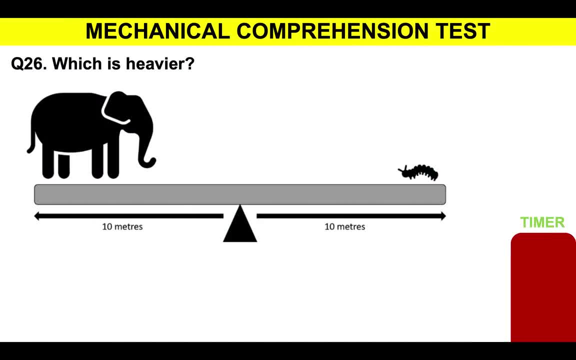 try one A. mechanical comprehension test, question 26.. Which is heavier? Is it A, an elephant B, caterpillar C? both the same Or D? cannot say. Now you'll see that the elephant and the caterpillar are on a seesaw here And that's the pivot and that's the distance there. 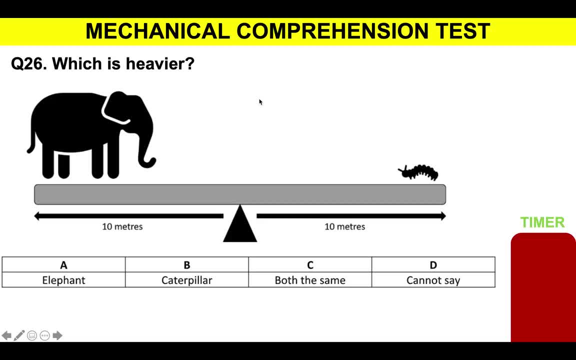 That is an important part of the question. Here's your timer. You have the time It takes the timer to go down to come up with your answer. Here we go, And I hope you didn't get caught out by that one. Now the next thing to do, because you're making brilliant.